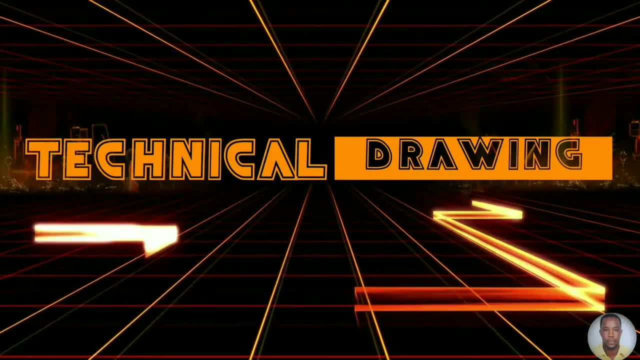 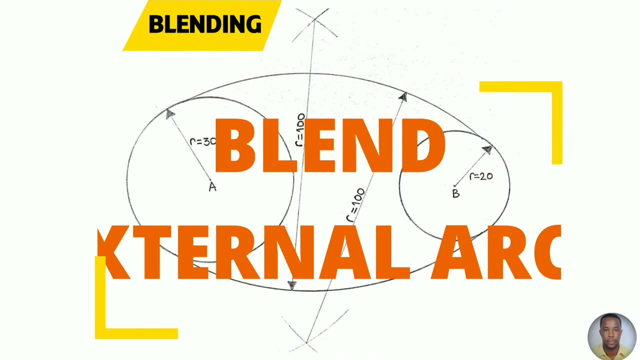 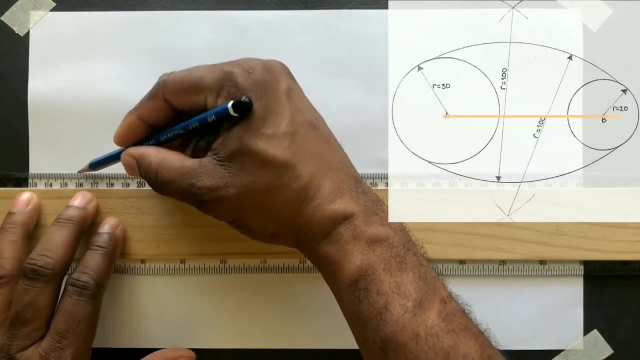 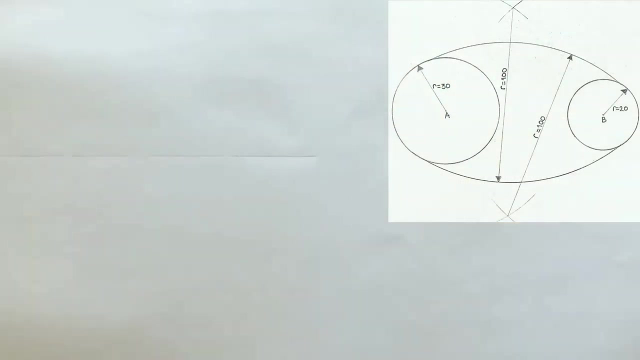 Greetings everyone. Sir Morgan, here from the technical department, From the topic blending arcs and circles, you will learn to blend an external arc to two circles. First, draw a horizontal centerline. Now measure 90 millimeters and identify these points on this line. 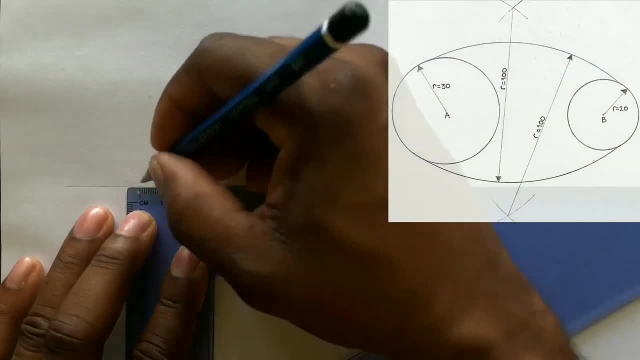 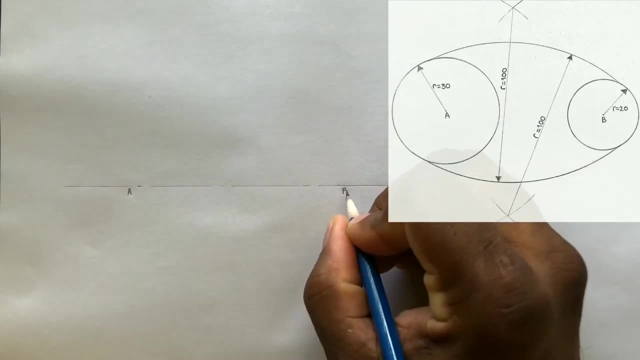 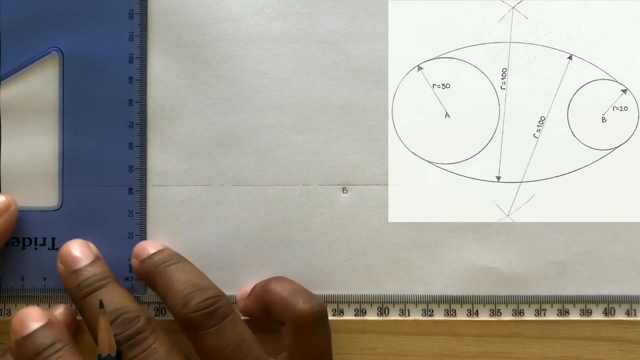 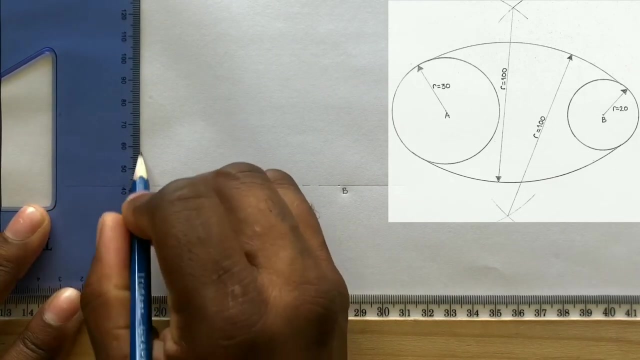 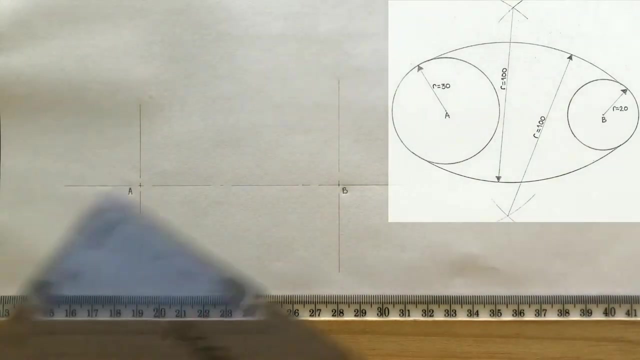 Label the points A and B. Use your T-square along with your C-square to mark the points A and B. Use your T-square along with your C-square to mark the points A and B. ji From A, draw a circle of radius 30 millimeters. 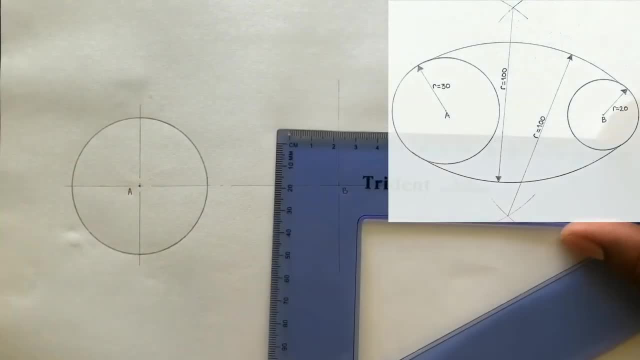 From B, draw a circular line of 30 millimeters from the perspective of the centerline. From B, draw a circular line of radius 30 millimeters from the perspective of the centerline. draw a circle of radius 20 millimeters. 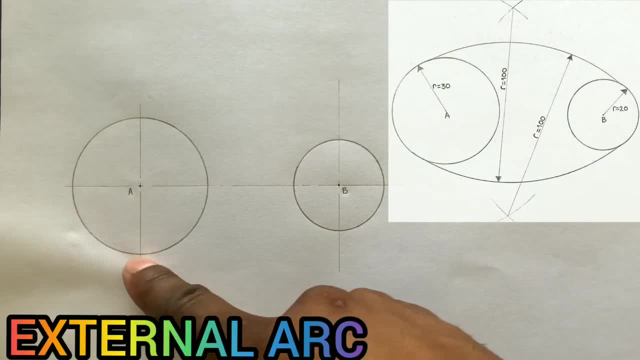 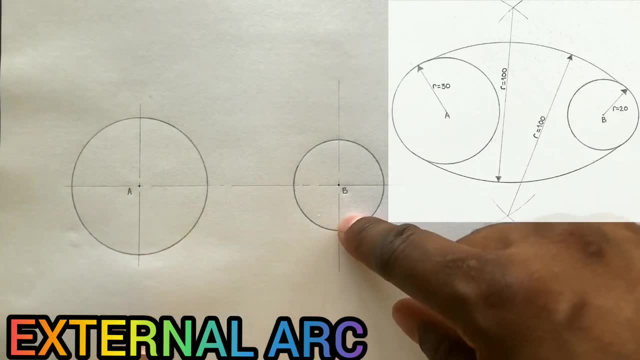 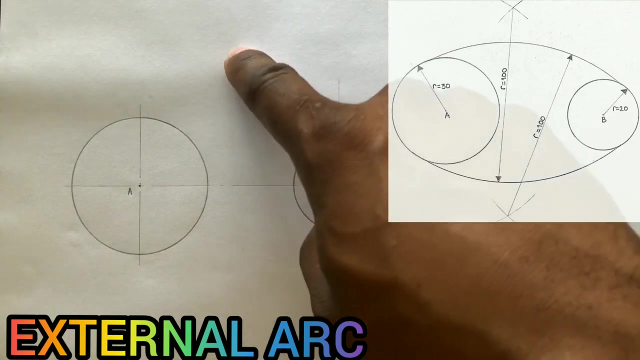 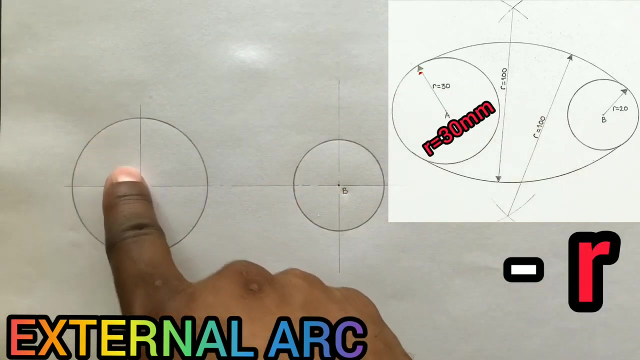 Now we need to draw an external arc to blend on these two circles. The radius given for this external arc is 100 millimeters. Now we need to first identify an intersection of arcs here to draw these two arcs. Now subtract 30 millimeters, which is this radius, from 100 millimeters, which is the external. 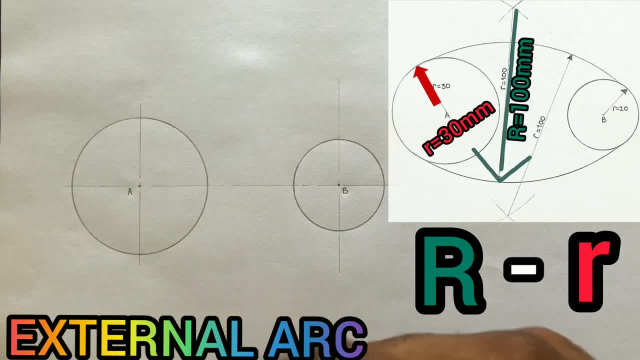 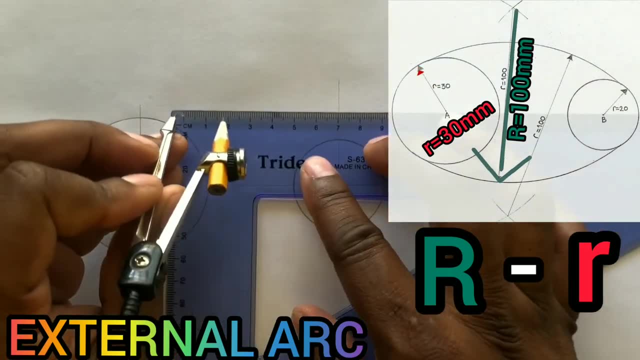 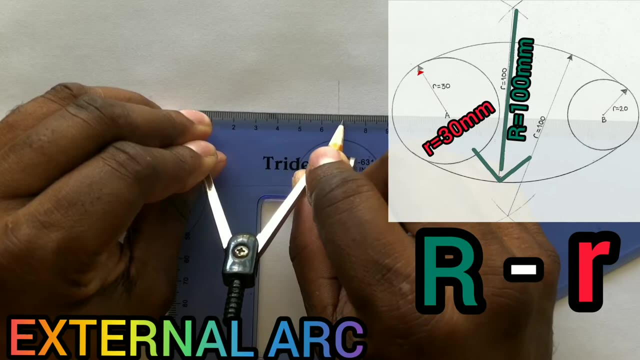 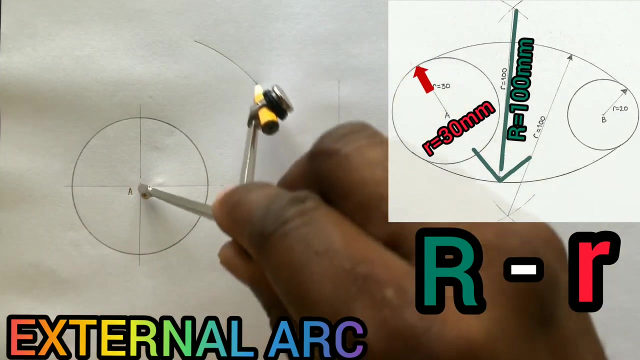 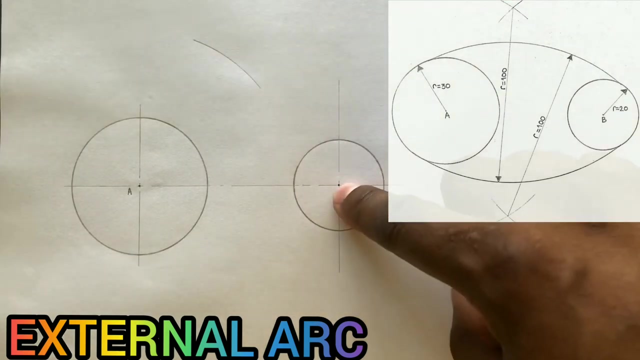 arcs radius 100 minus 30, equal to 70.. Open your computer, compass to 70 millimeters and, from the center, a scribe, an arc. Now we need to get another arc to intersect this arc from this center. Now, subtracting this, 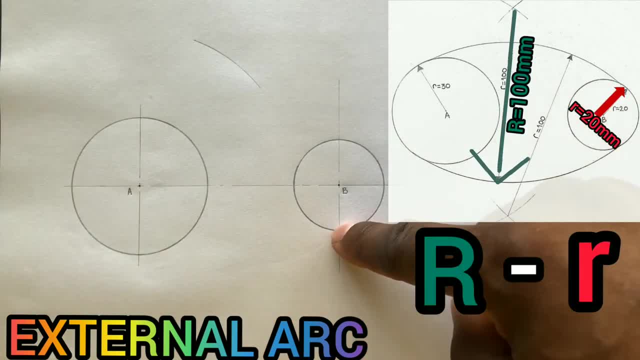 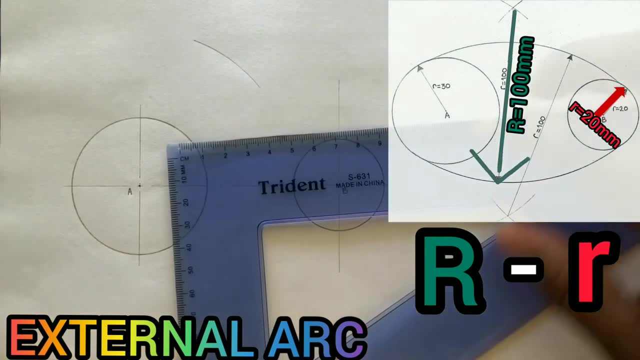 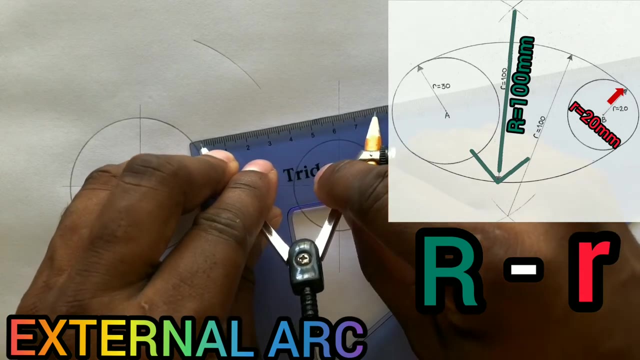 radius from the external arcs radius will give us 80.. Millimeters: 100 minus 20 millimeters equals 20 millimeters equals 80 millimeters. Open your compass to a radius of 80 millimeters. Now, from B scribe an arc. 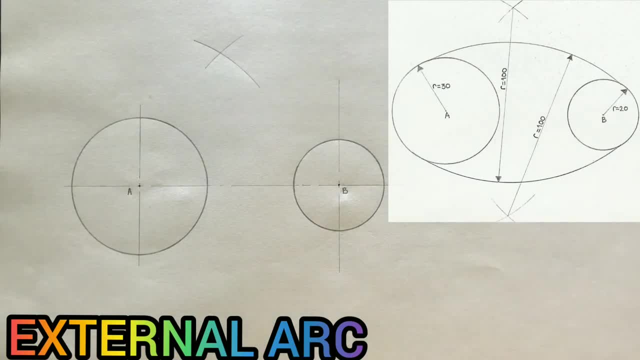 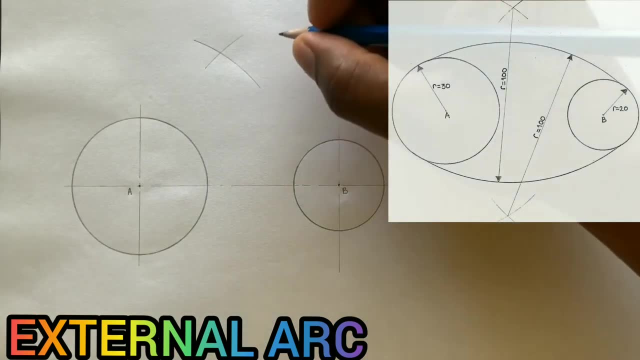 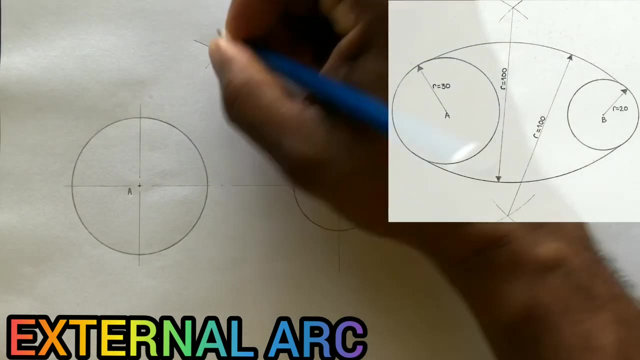 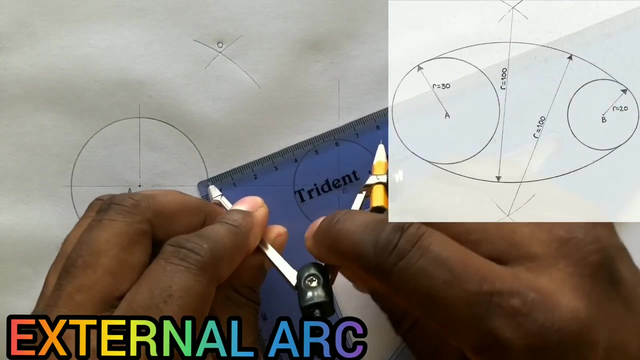 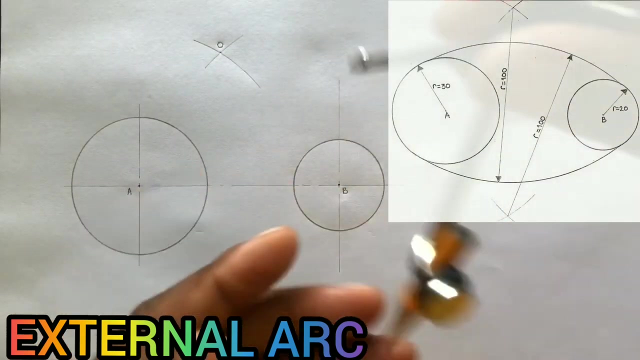 Now from the intersection of arc. we will draw our external arc here. Identify and label these intersections as: O. Now open your compass to a radius of 100 millimeters. This 100 millimeters is a given radius. Now draw your external arc from the center. O. 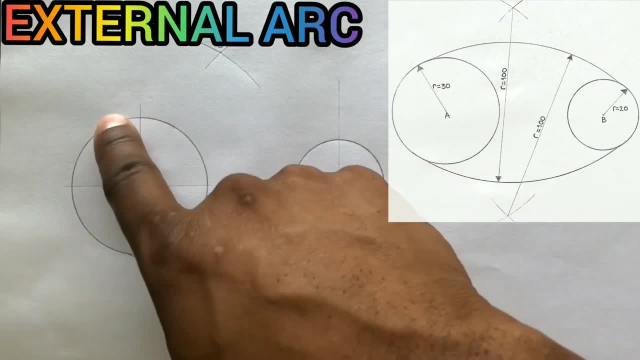 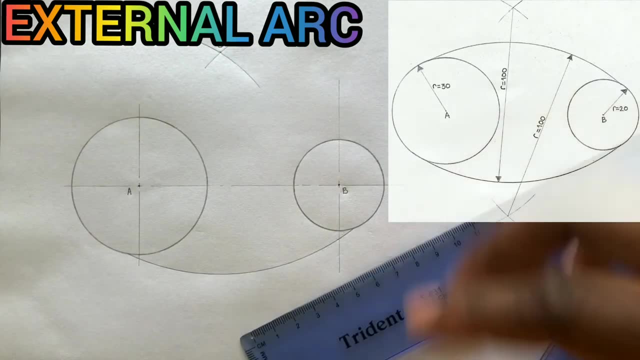 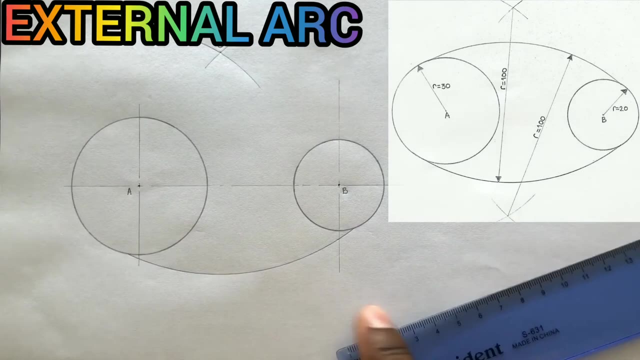 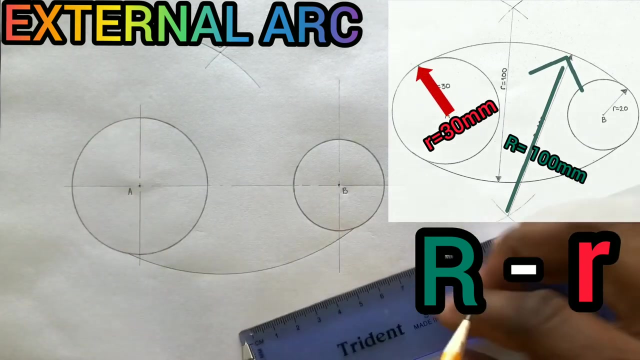 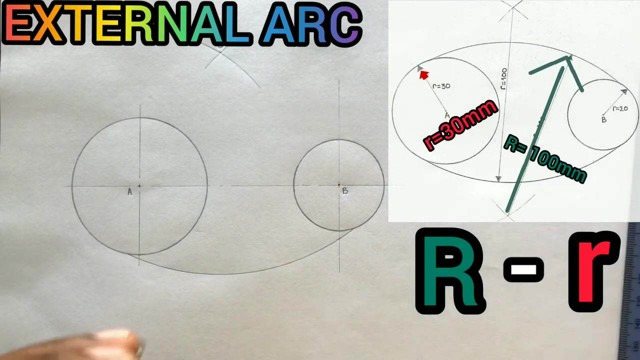 There you go. Now we could do the same procedure to get another external arc here. Open your compass to a radius of 70 millimeters. Now this 70 millimeters is the radius of the external arc minus the radius of this circle. Now from A scribe, 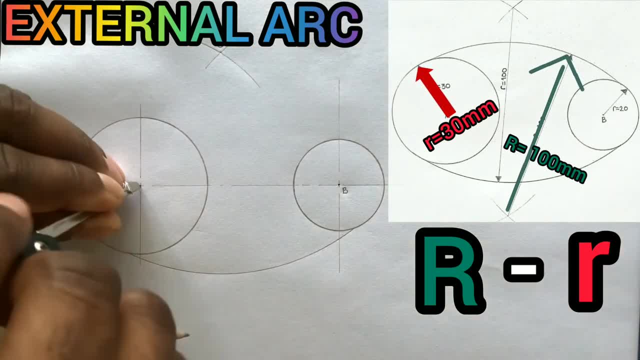 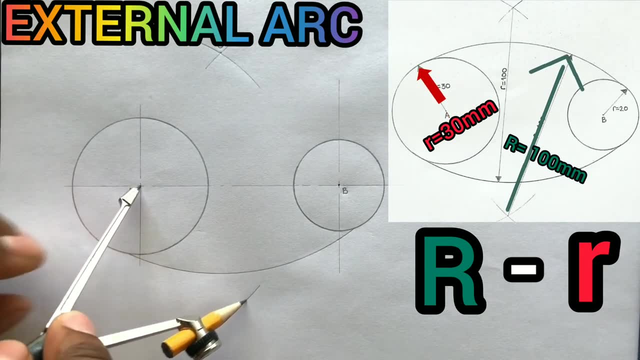 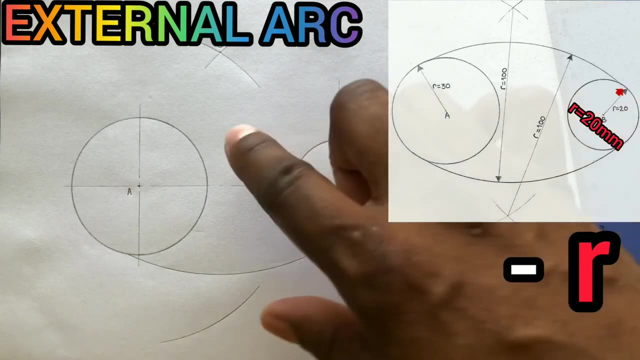 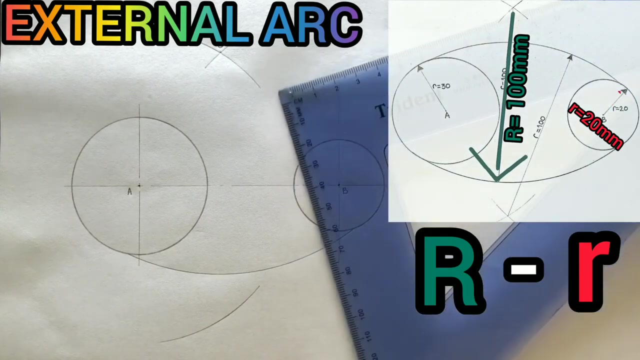 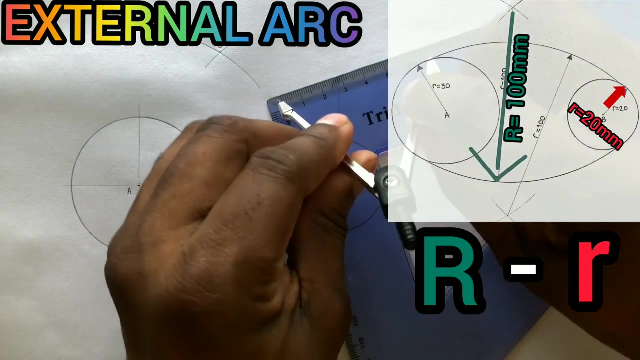 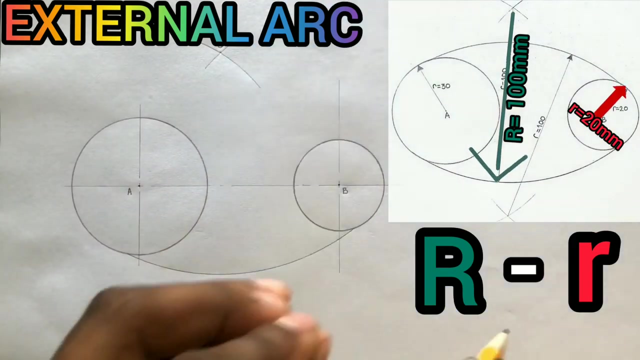 an arc below the two circles. Now, with the same procedure, you will subtract 20 millimeters from the external arc of 100 millimeters, giving you 80 millimeters. Open your compass to 80 millimeters, Open theаютing print functionpt Mina and from B scribe an arc. 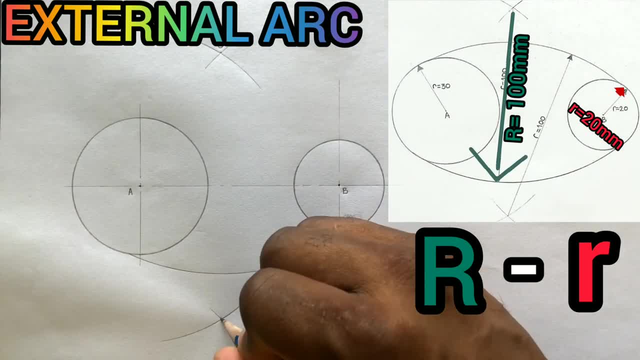 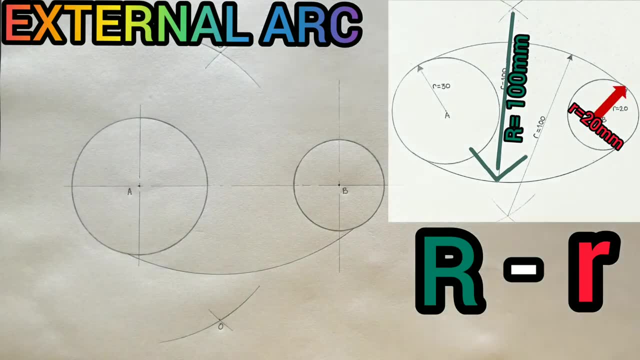 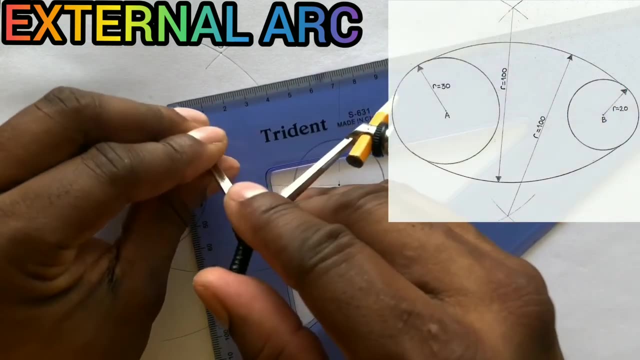 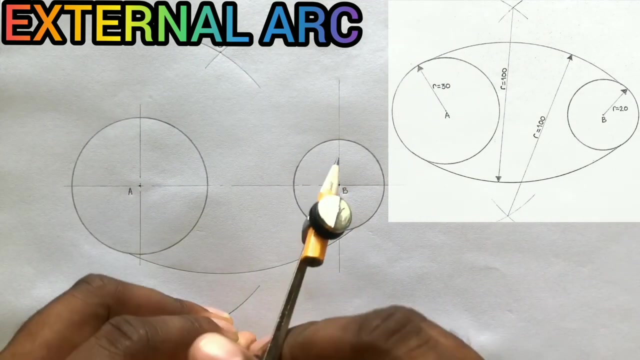 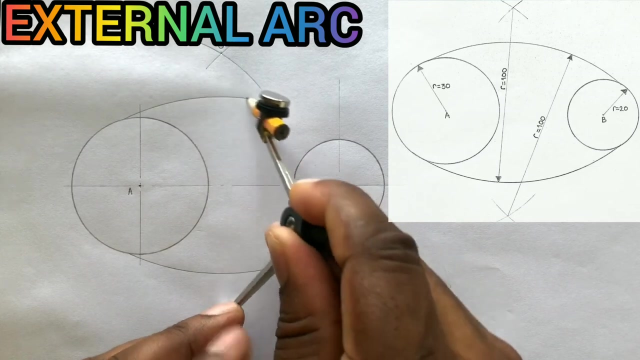 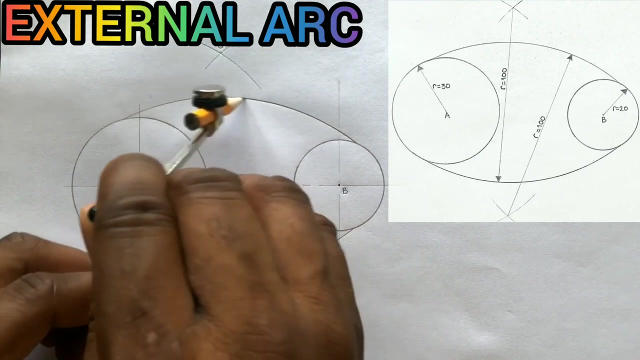 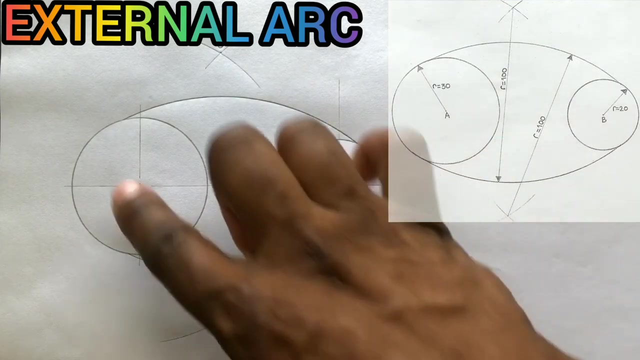 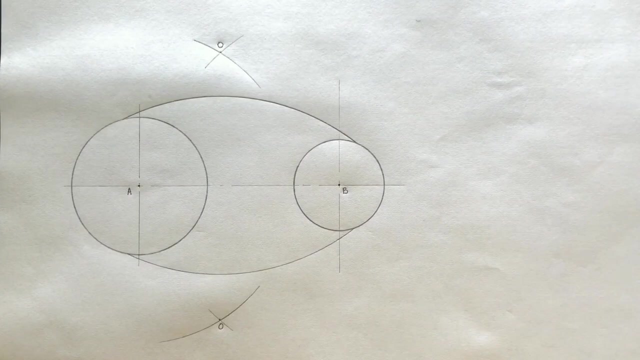 Label this intersection of arc as O. Now open your compass to a radius of 100 millimeters and from this center, O draw your external arc. so there you go. now to these two circles. you have just constructed two external arcs border your paper and complete your title block. so you.